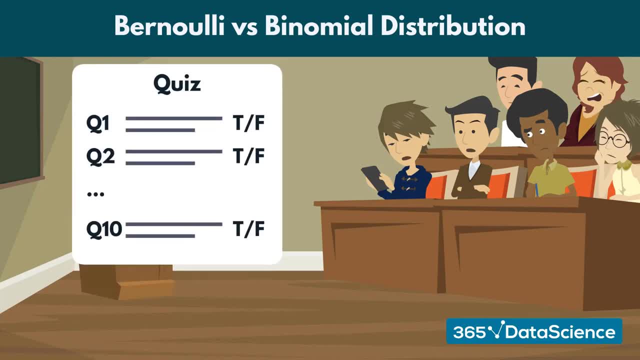 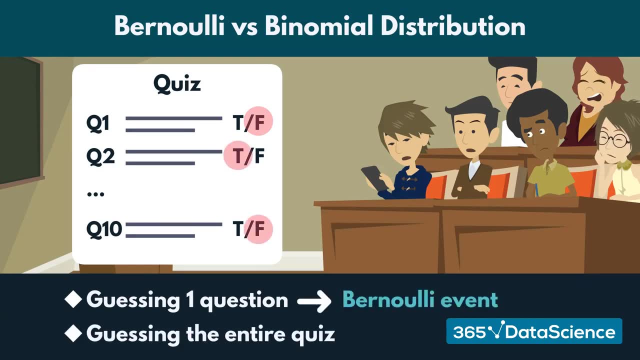 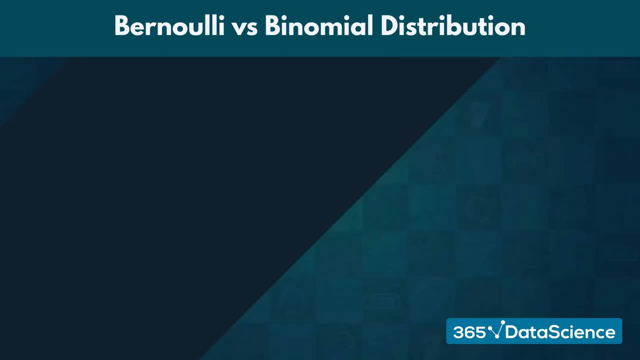 Luckily for you, the quiz consists of 10 true or false questions. In this case, guessing a single true or false question is a Bernoulli event, but guessing the entire quiz is a binomial event. Alright, let's go back to the quiz example we just mentioned. 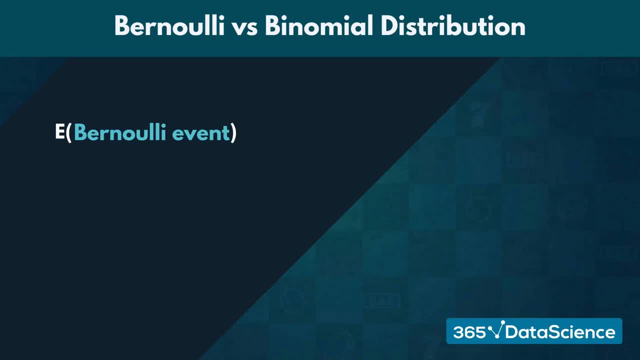 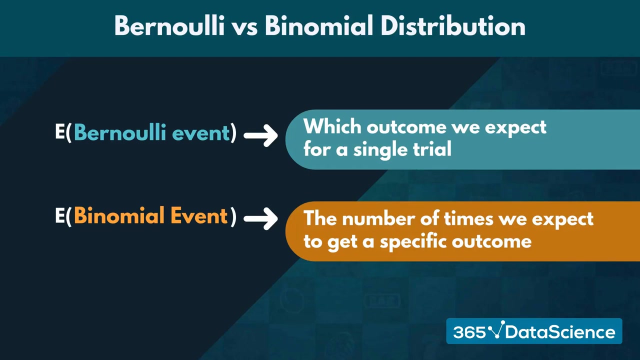 In it. the expected value of the Bernoulli distribution suggests which outcome we expect for a single trial. Now, the expected value of the binomial distribution would suggest the number of times we expect to get a specific outcome. Great, Now, the graph of the binomial distribution represents the likelihood of attaining our 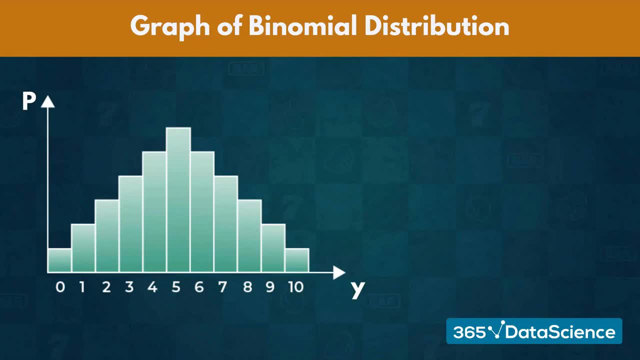 desired outcome a specific number of times. If we run n trials, our graph would consist n plus 1, many bars, one for each unique value, from 0 to n. For instance, we could be flipping the same unfair coin we had from the last lecture. 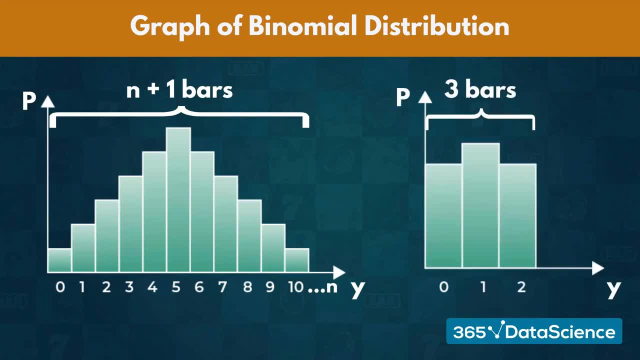 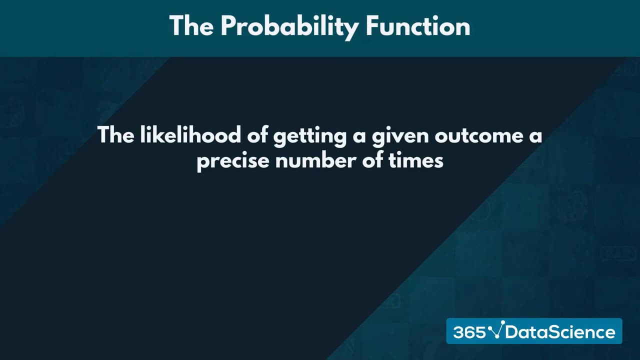 If we toss it twice. we need bars for the three different outcomes: 0,, 1, or 2 tails Fantastic. If we wish to find the associated likelihood of getting a given outcome a precise number of times over the course of n trials, we need to introduce the probability function of the 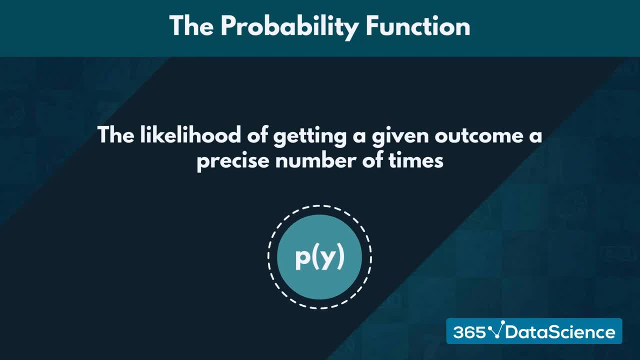 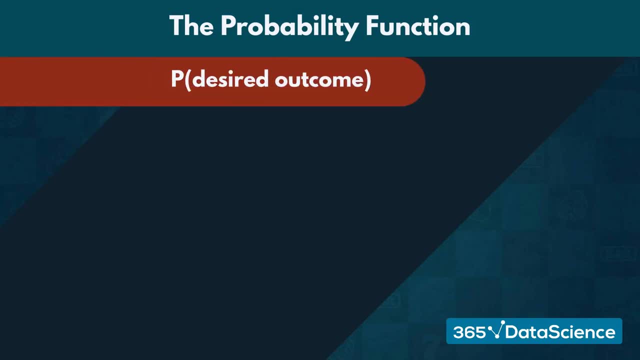 binomial distribution For starters. For starters, each individual trial is a Bernoulli trial, so we express the probability of getting our desired outcome as p and the likelihood of the other one as 1 minus p. In order to get our favored outcome exactly y, many times over the n trials, we also need 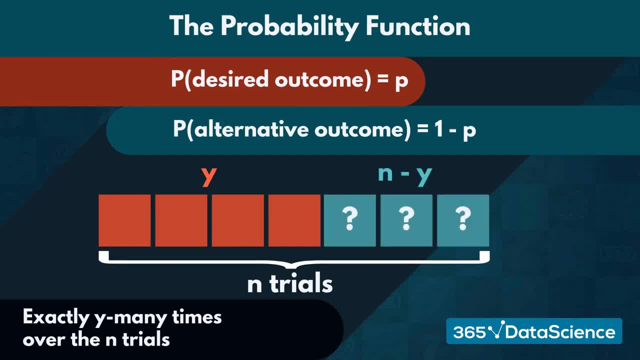 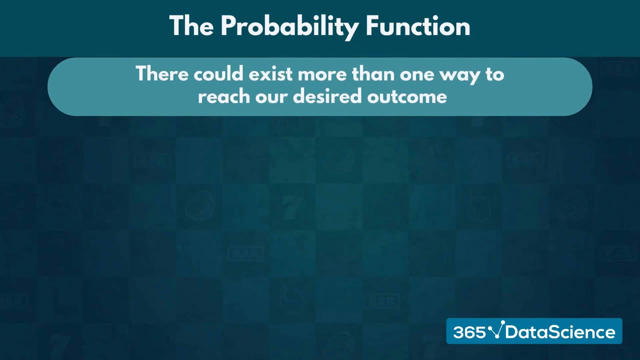 to get the alternative outcome n minus y many times. If we don't account for this, we would be estimating the likelihood of getting our desired outcome at least that n times. Additionally, more than one way to reach our desired outcome could exist. To account for this, we need to find the number of scenarios in which y out of the n many. 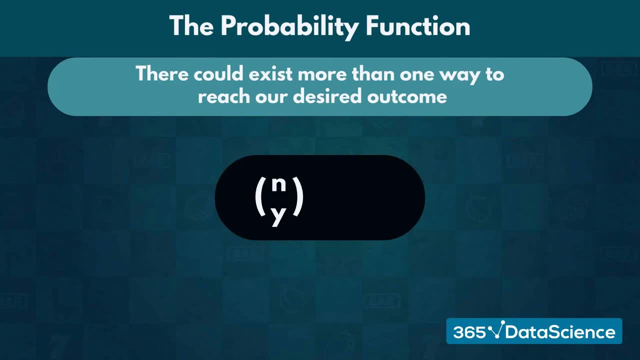 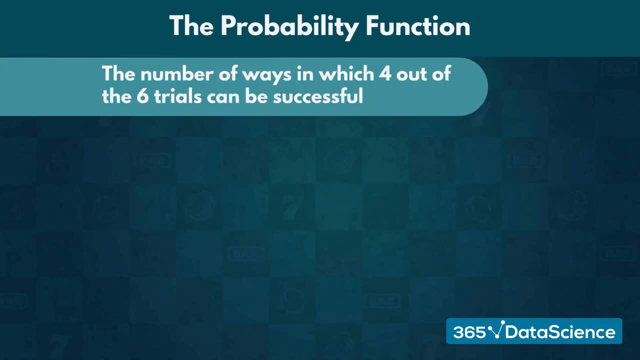 outcomes would be favorable, But these are actually the combinations we already know. For instance, if we wish to find out the number of ways in which four out of the six trials could be successful, it is the same as picking four elements out of a sample space of 4.. 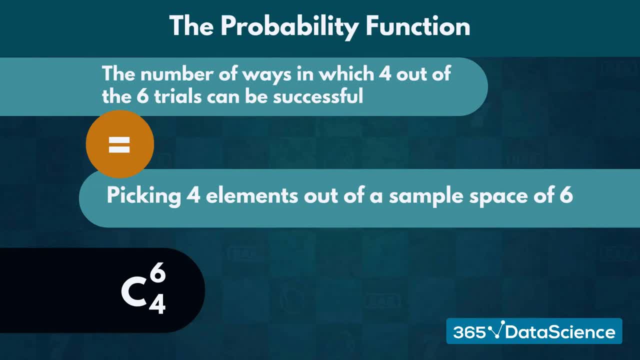 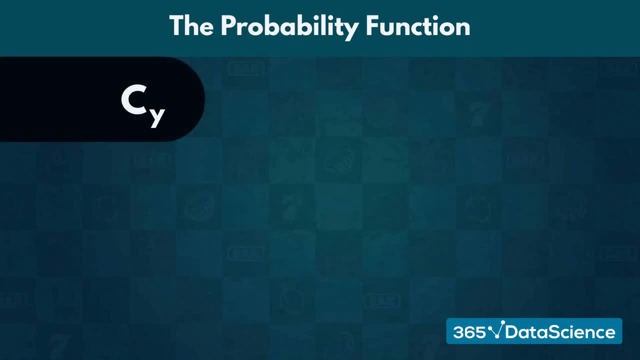 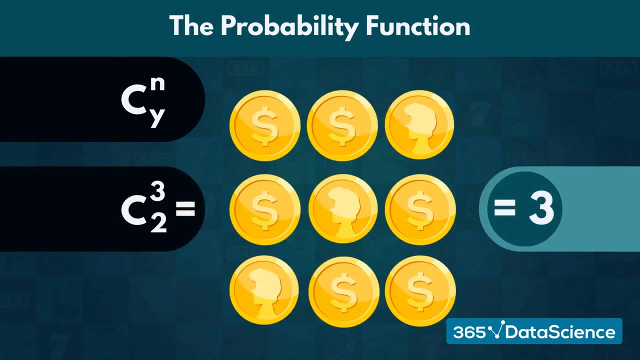 of 6.. Now you see why combinatorics are a fundamental part of probability. Thus, we need to find the number of combinations in which y out of the n outcomes would be favorable. For instance, there are three different ways to get tails exactly twice in three coin. 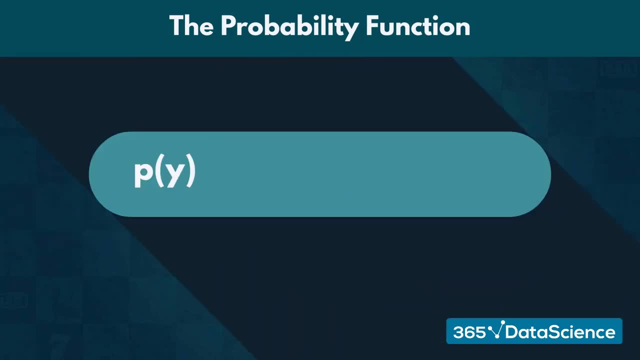 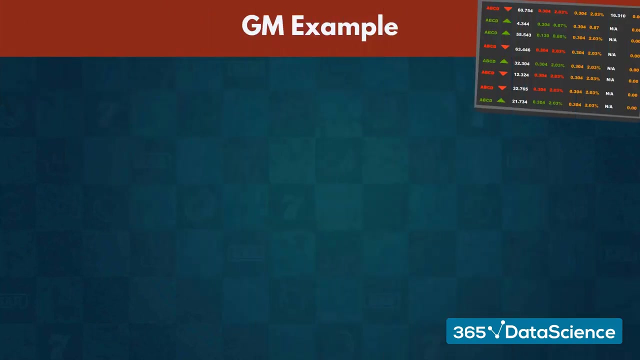 flips. Therefore, the probability function for a binomial distribution is the product of the number of combinations of picking y many elements out of n times p to the power of y, times 1-p to the power of n-y. Great To see this in action. let us look at an example. 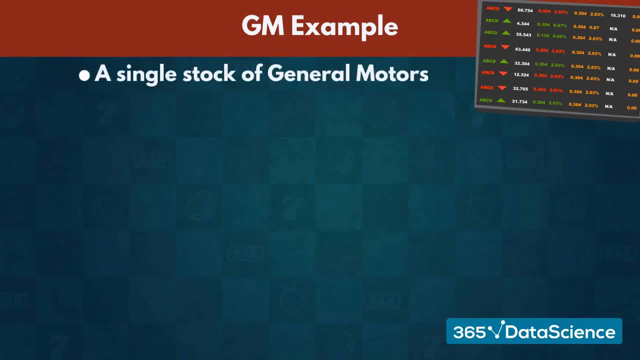 Imagine you bought a single stock of General Motors. Historically you know there is a 60% chance the price of your stock will go up on any given day and a 40% chance it will drop. So there is a 60% chance it will drop on any given day And there is a 30% chance that. 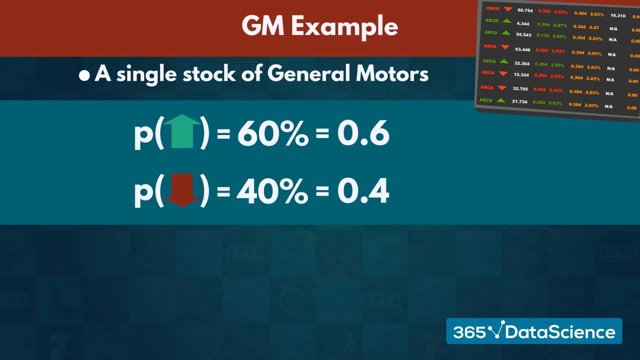 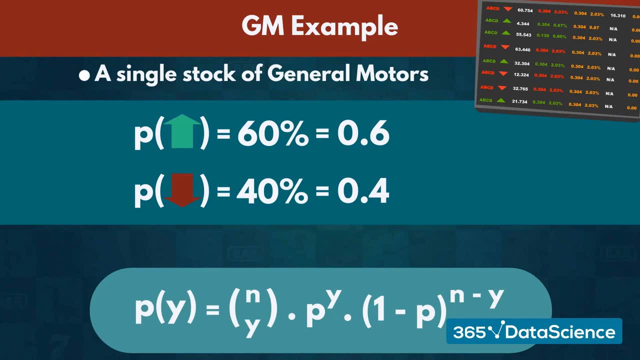 or 40% chance that the price of your stock downstairs Will drop- who knows how fast it. By the price going up we mean that the closing price is higher than the opening price. With the probability distribution function you can calculate the likelihood of the stock price increasing 3 times during the 5 workday week. 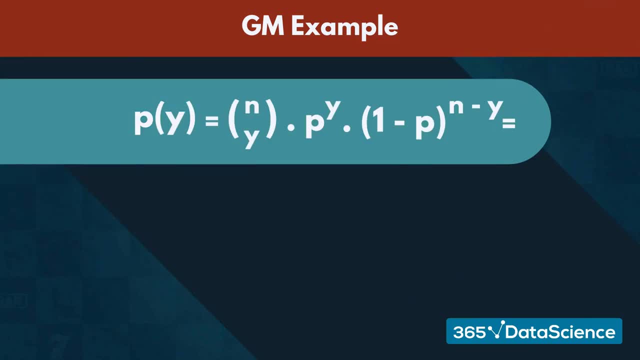 If we wish to use the probability distribution formula, we need to plug in 3 for Y, 5 for N and 0.6 for P. After plugging in, we get Number of different possible combinations of picking 3 elements out of 5 times 0.6 to the power of 3 times 0.4 to the power of 2.. 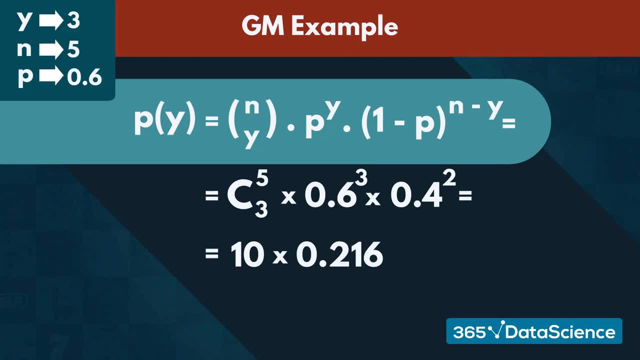 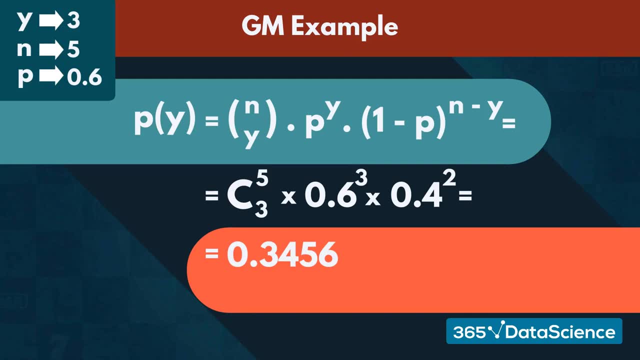 This is equivalent to 10 times 0.216 times 0.16 or 0.3456.. Thus, we have a 34.56% chance of getting exactly 3 increases over the course of a week. The big advantage of recognizing the distribution is that you can simply use these formulas and plug in the information you already have. 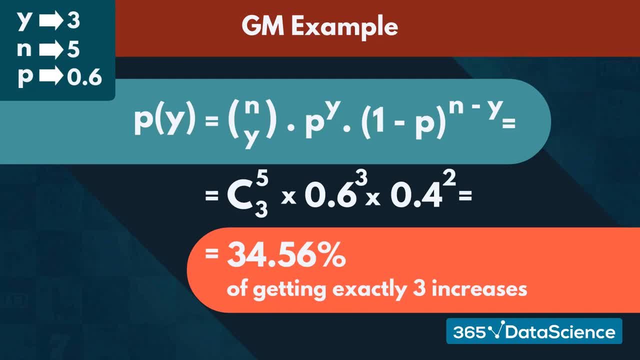 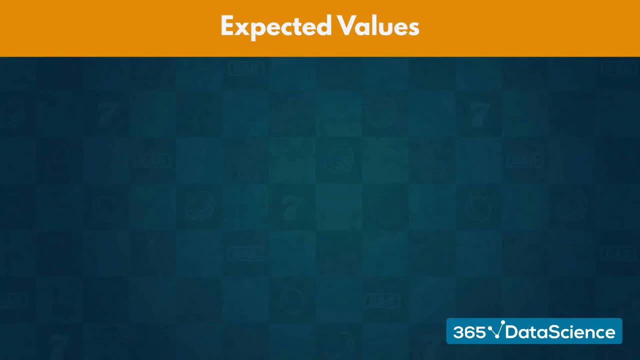 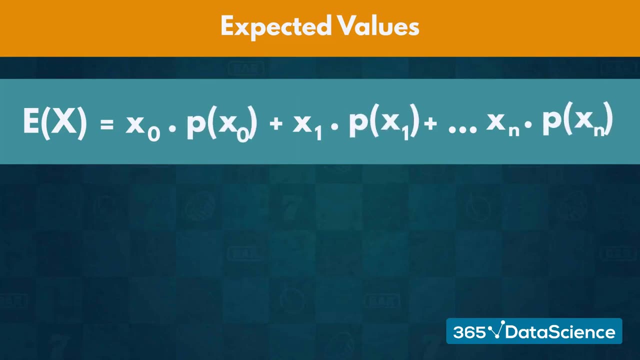 Alright, now that we know the probability function, we can move on to the expected value. By definition, the expected value equals the sum of all values in the sample space multiplied by their respective probabilities. The expected value formula for a binomial event is the following: